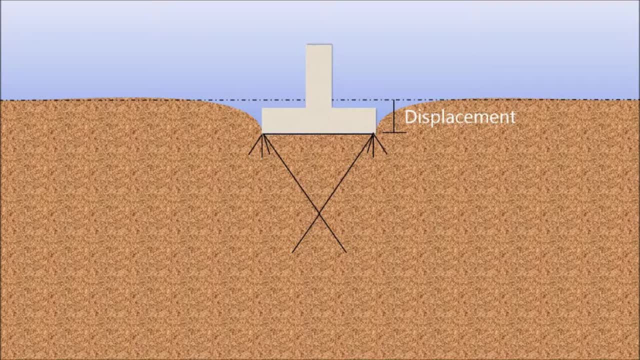 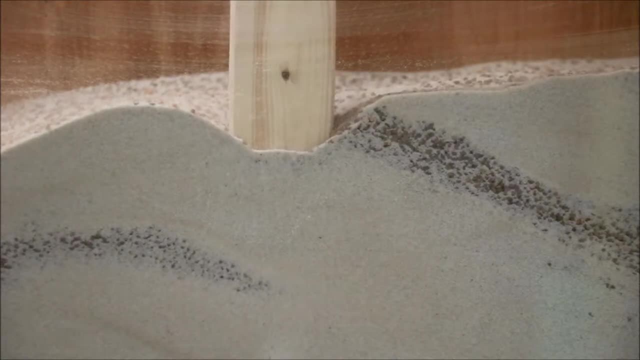 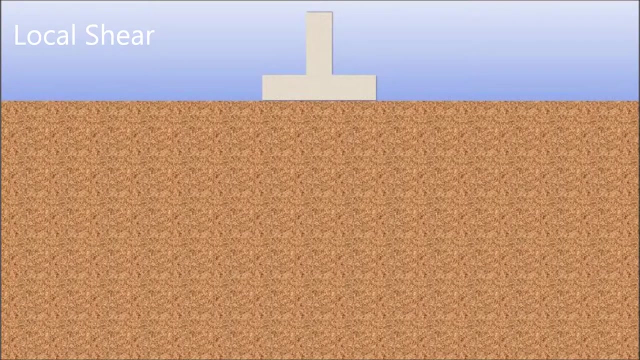 slowly. Failure develops gradually in this setting due to the high compressibility of these soils. Little to no soil disturbance is seen at the surface when punching shear occurs, but structures experience high levels of settlement. Local shear failure occurs in cohesionless and loose to medium dense soils. This failure mode has a well-defined shear surface directly under the. 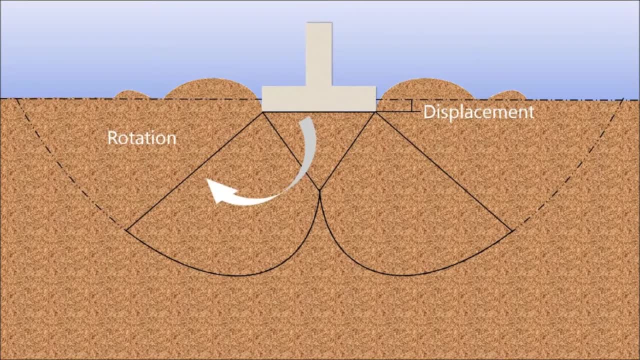 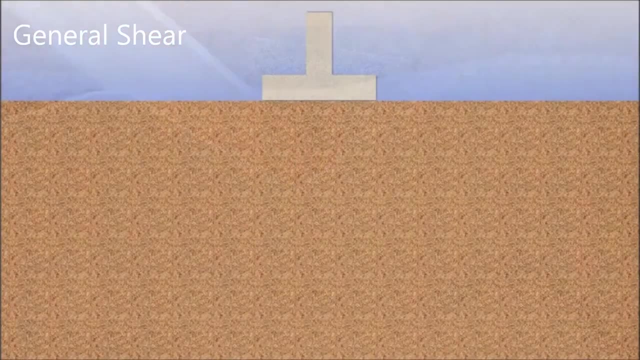 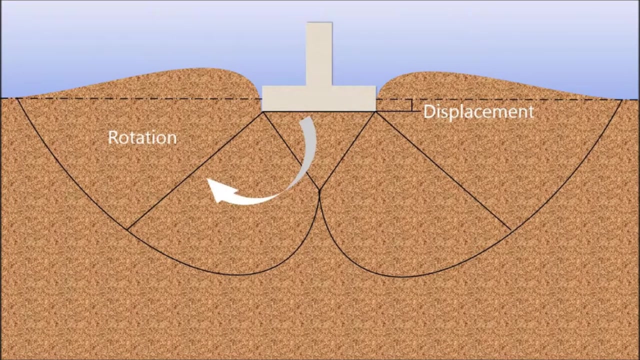 footing that may or may not be seen at the surface of the soil. Local shear failure happens gradually as the footing continues to experience settlement and movement along the shear plane. General shear failure occurs in dense, cohesionless soils and undrained cohesive soils. General shear failure. 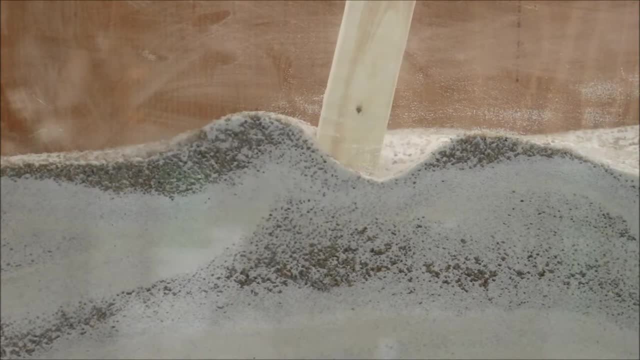 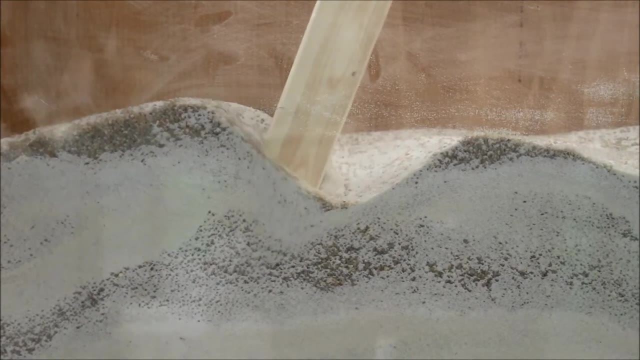 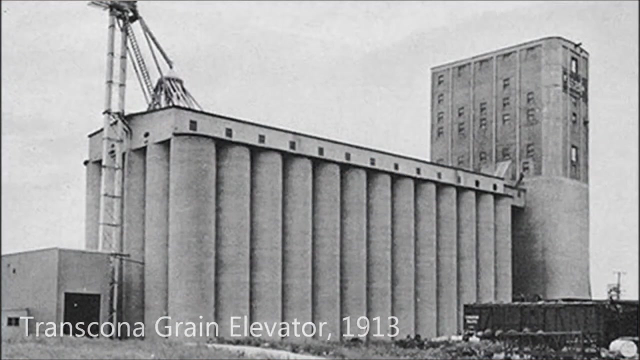 is characterized by a well-defined shear plane with clearly formed disturbances in the surface of the soil. Local shear failure occurs suddenly and can cause significant rotation of the structure. Over the years, there have been several extreme instances of bearing capacity failure. One historic event involved the Transcona Grain Elevator constructed in Manitoba, Canada. The 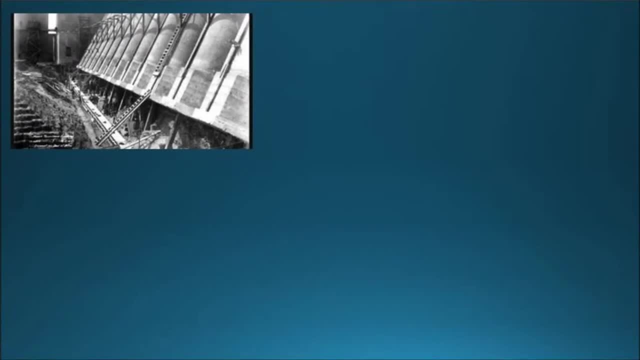 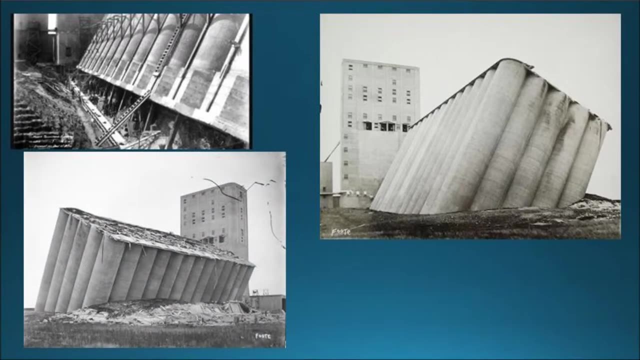 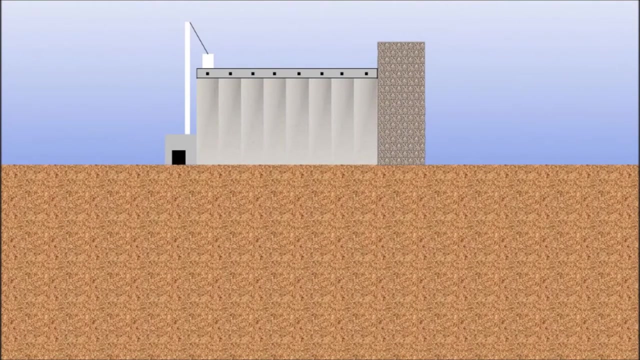 elevator design had overestimated the bearing capacity of the soil and underestimated the load from the grain. This led to the structure experiencing a sudden and dramatic general shear failure. Engineers have developed methods to safely support shear failure in the soil, support structures and transfer loads in soils with low or insufficient bearing capacities. 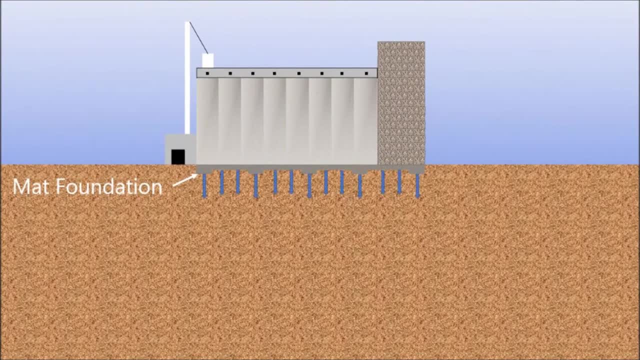 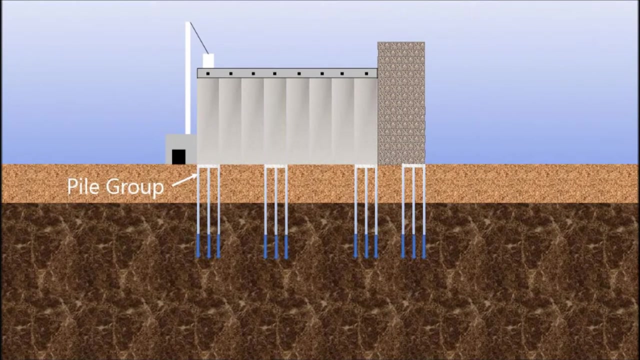 One method is to distribute the load of the structure over a larger surface area. Mat and raft foundations are used for this application and usually span the entire footprint of the structure they support. Another option is to bypass weak soil layers and transfer loads to stronger layers or even bedrock below. This is accomplished with deep foundations. There are 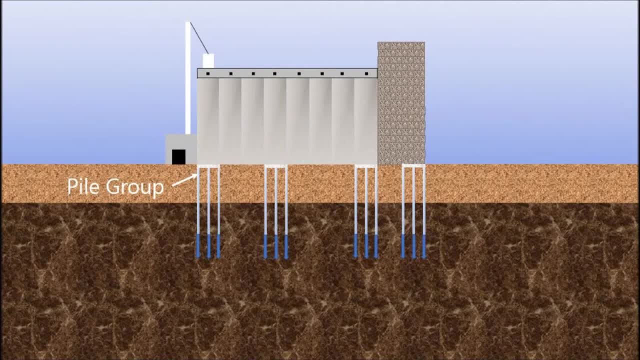 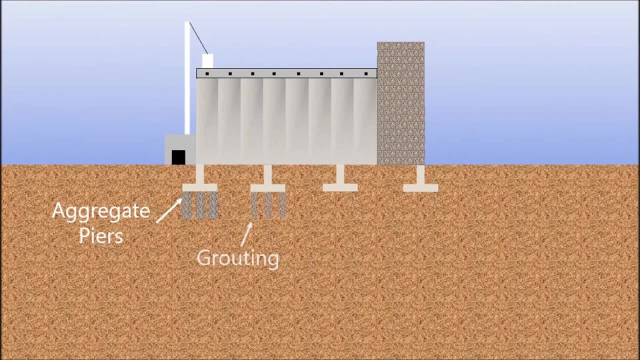 several types of deep foundations, which are generally categorized as driven piles, drilled shafts and auger piles. Soil improvement can also be used with shallow foundations to get the necessary strength for structural support. Soil improvement technologies strengthen and reinforce existing soil structures at sites to increase bearing capacity. There are many. 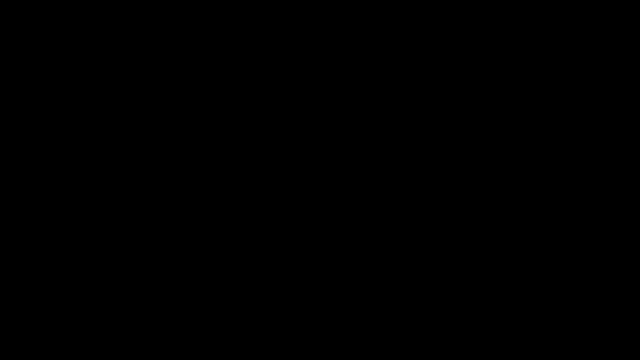 different options for soil improvement, with new technologies being developed regularly.